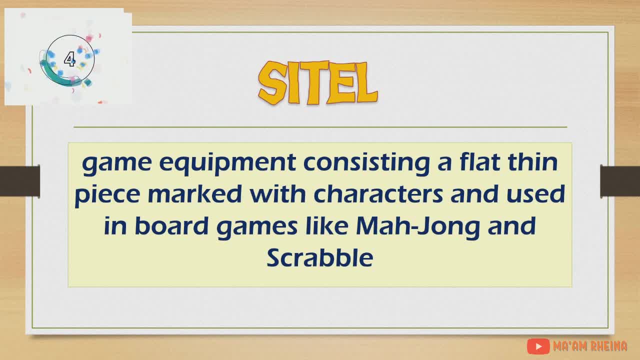 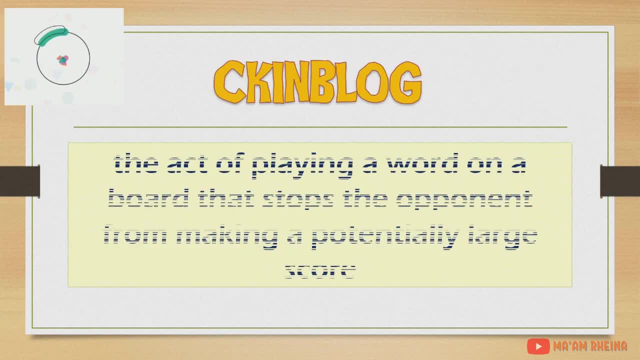 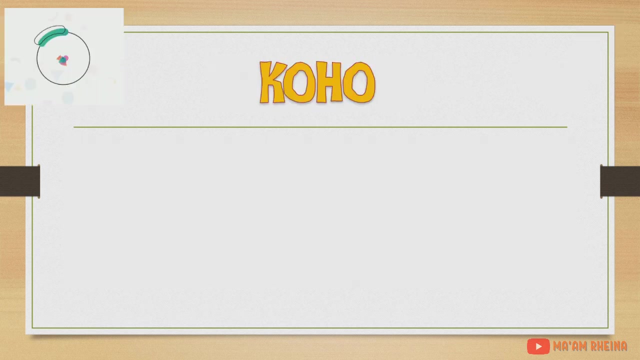 games like Mahjong and Scrabble. Well done, The word is tiles. Next, The act of playing a word on a board that stops the opponent from making a potentially large score. Correct again, The answer is blocking Next term A letter that will spell a new word when it is played with in the front or at the end. 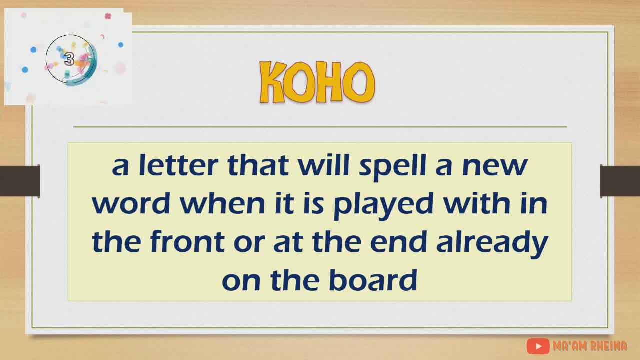 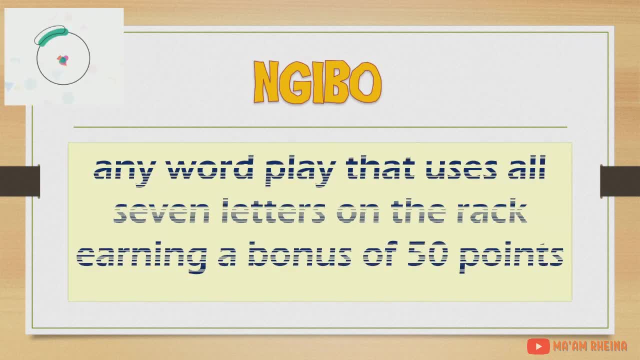 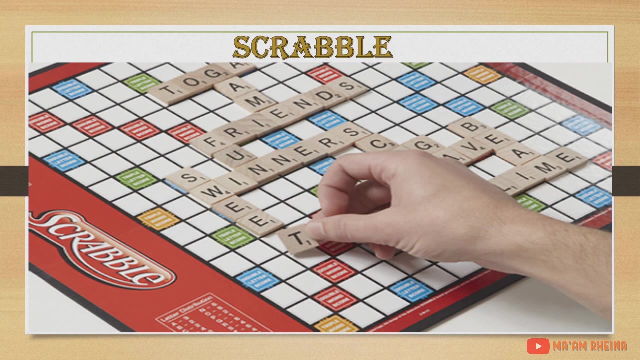 already on the board. That is right, It's hook. Next, Any word play that uses all seven letters on the rack, earning a bonus of 50 points. Great job, Bingo is the correct answer. Now let us discuss the next term: A letter that will spell a new word when it is played with in the front or at the end, already on the board. That is right, It's hook. Next term, A letter that will spell a new word when it is played with in the front or at the end, already on the board. That is right, It's hook. 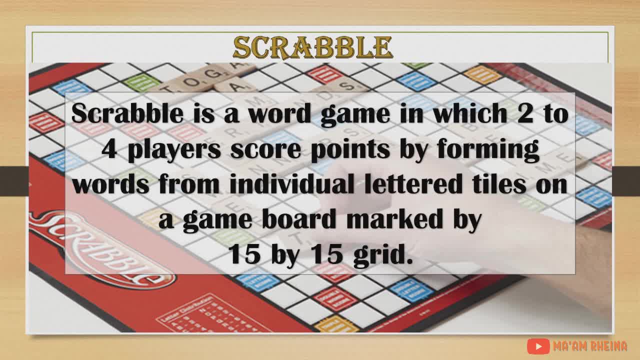 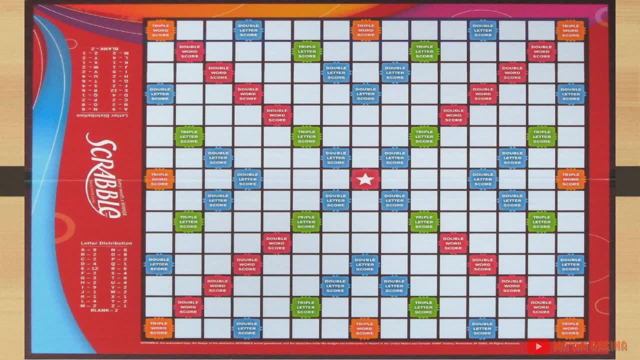 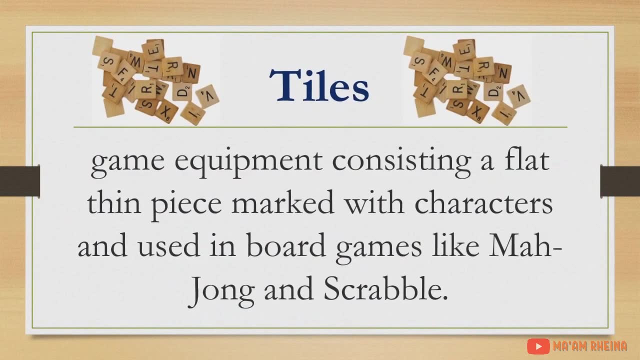 Scrabble. Scrabble. Scrabble is a word game in which two to four players score points by forming words from individual lettered tiles on a game board marked by 15 by 15 grid. This is an example of a Scrabble board. It has 15 by 15 grid with a star square at the center. Tiles, Game equipment. 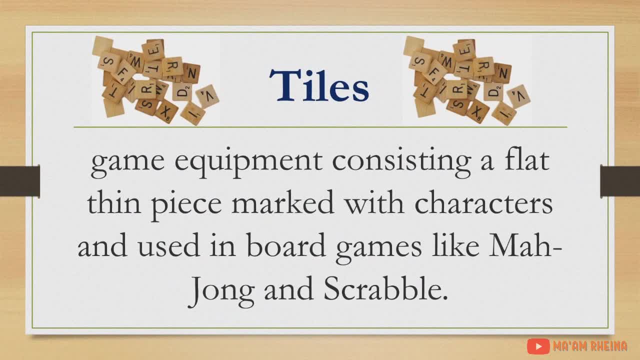 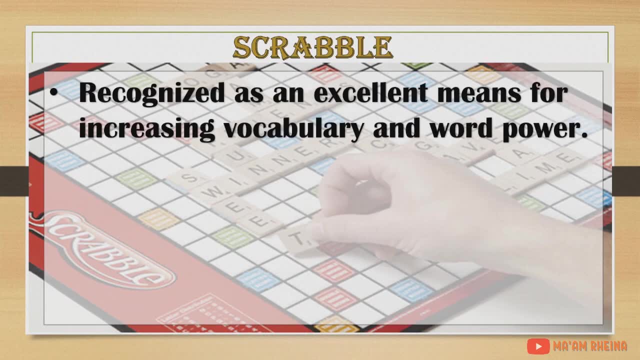 consisting of flat, thin piece marked with characters and used in board games like Mahjong and Scrabble. These are all we need in playing this game. Scrabble is recognized as an excellent means of playing this game. Scrabble is recognized as an excellent means for a new player to play. 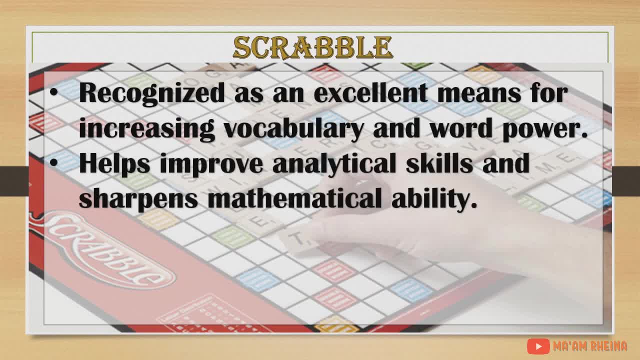 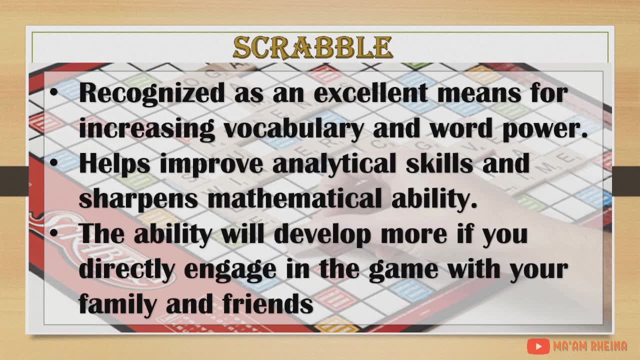 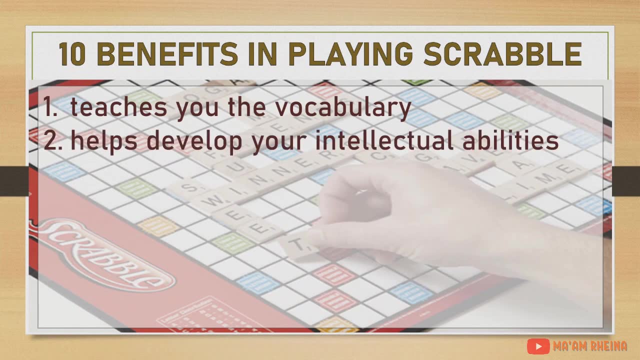 for increasing vocabulary and word power. It helps improve analytical skills and sharpens mathematical ability. The ability will develop more if you directly engage in the game with your family and friends. 10 Benefits in Playing Scrabble: Scrabble teaches you the vocabulary. It helps develop your intellectual abilities. 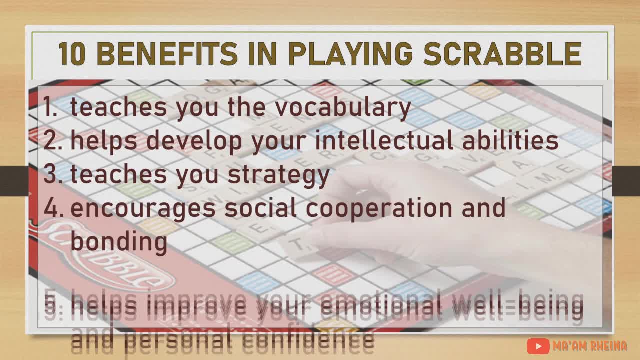 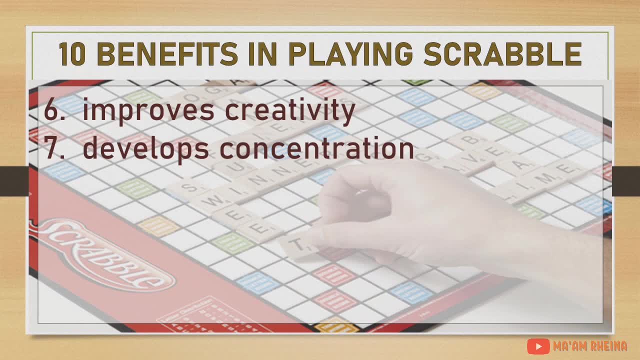 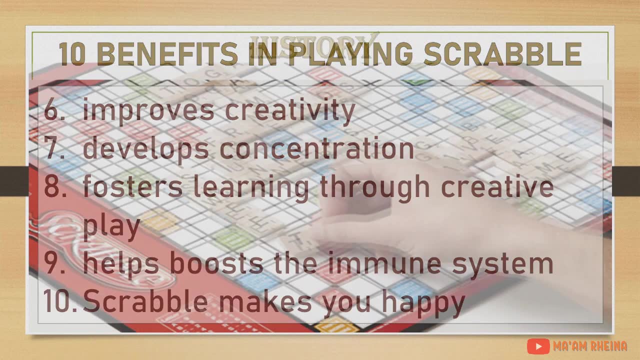 teaches you strategy, encourages social cooperation and bonding. helps improve your emotional well-being and personal confidence, improves creativity, develops concentration, fosters learning through creative play, helps boost the immune system and Scrabble makes you happy. Originally called Criss-Cross, the game, which was based on the crossword puzzle and 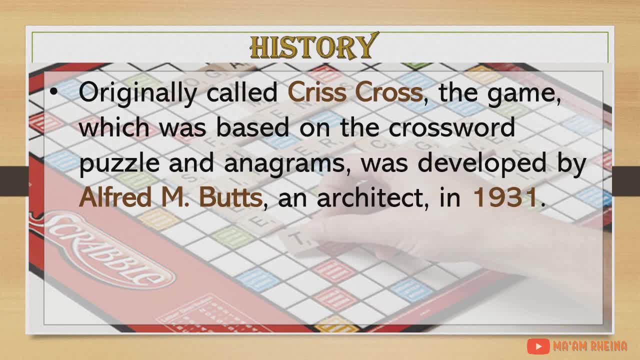 anagrams was developed by Alfred M Butts, an architect, in 1931.. It was redesigned, renamed as Scrabble and marketed by James Bruno in 1948.. It was first sold in Great Britain in 1954.. 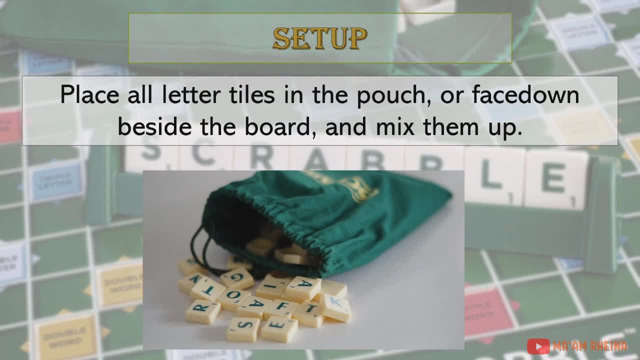 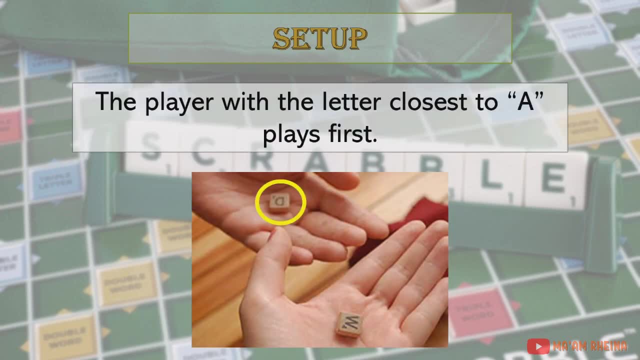 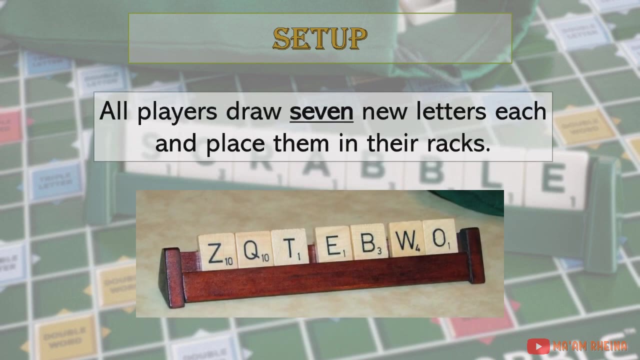 Setup of the game. Place all letter tiles in the pouch or face down beside the board and mix them up. Draw for the first play. The player with the letter closest to letter A plays first. A blank tile beats any letter. Return the letters to the pool and remix All players. draw seven new letters each and place. 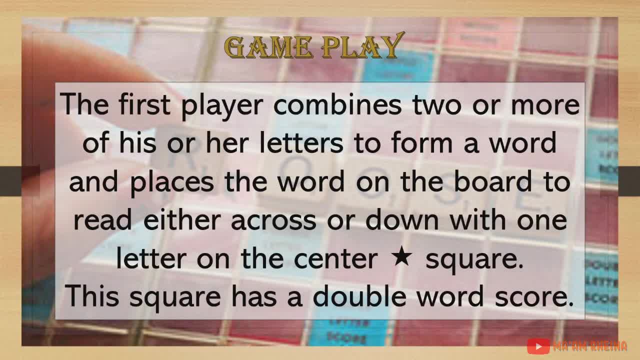 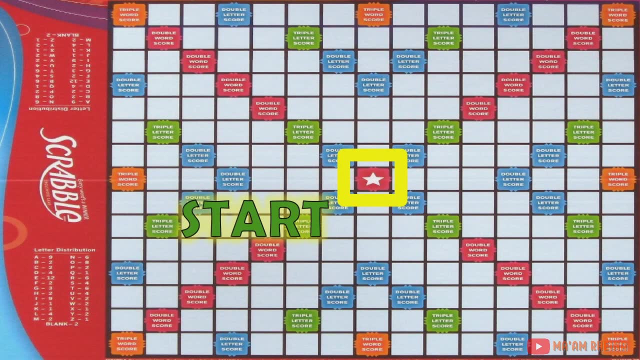 them in their racks. The first player combines two or more of his or her letters to form a word and a word on the board to read either across or down, with one letter on the center star square. This square has a double word score. This is the center star square. The first player can place a 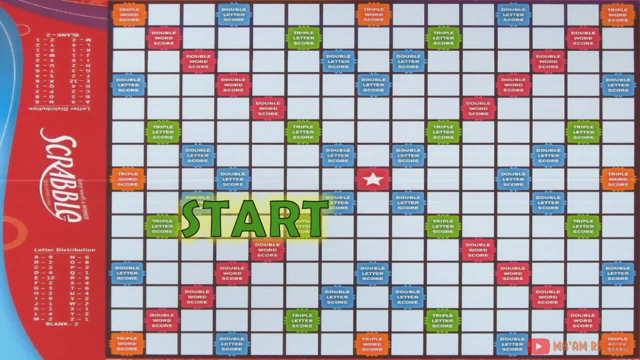 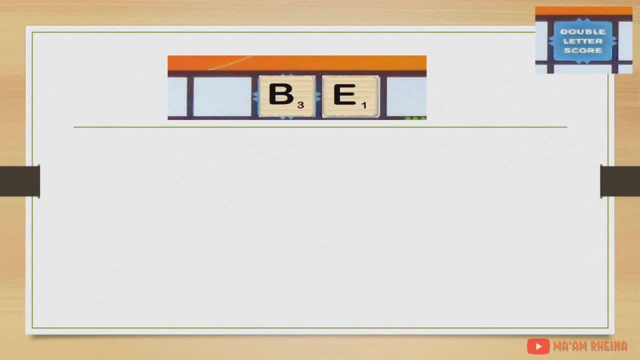 word, either across or down, with one letter on it. You can also see other squares with extra point values. Double letter score doubles the letter value, For example, for the word B. letter B has three point value and it is on the double letter score. Now multiply three points. 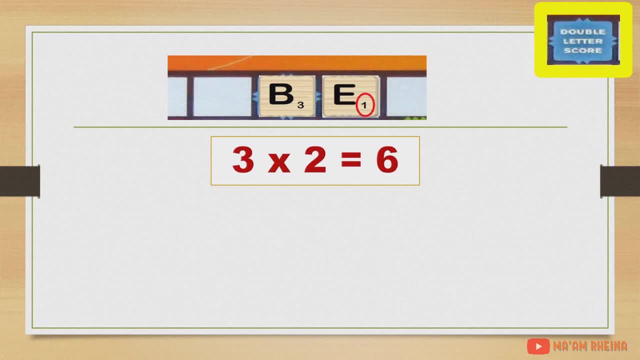 Add three by two to double the score of the letter B. It is equals to six. Then add the remaining letter value. E has one point. Six plus one equals seven. The score of the word played is seven. Triple letter score triples the letter value If the letter B for this word is placed. 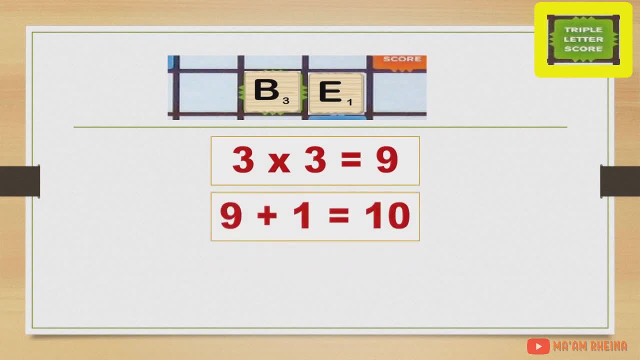 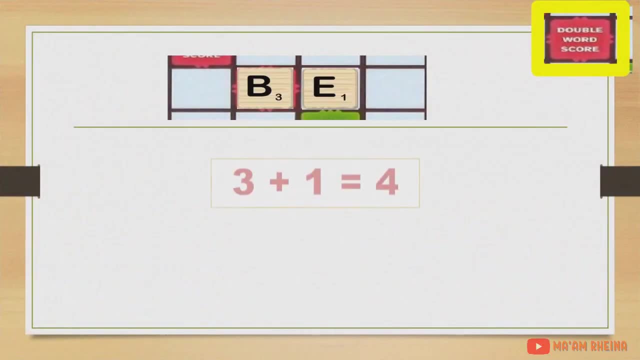 here. multiply the letter value by three, Then add the value of the remaining letter. Double word score doubles the points of the word played. If the same word is placed in this square, add the total point of the word. Then multiply it by two. And triple word score triples the value of the word. Add the total point. 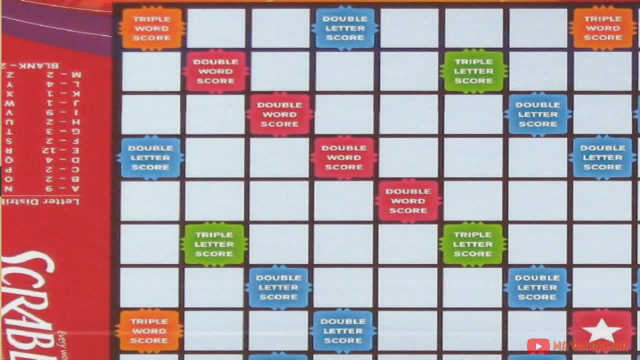 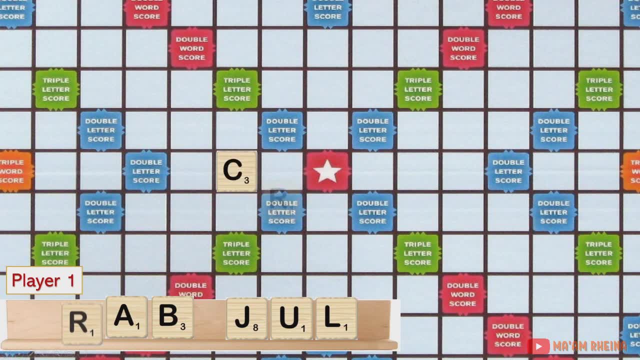 of the word and multiply it by three. The extra point squares on the board can only be used one time. Let us have an example. The first player placed his first word, crab. To compute his score, add the total point of each letter. Remember that the center star square has a double word score. 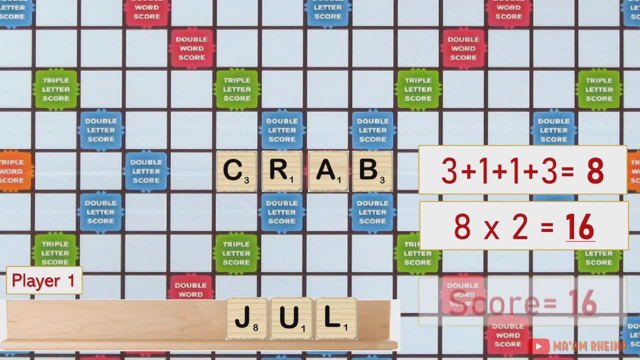 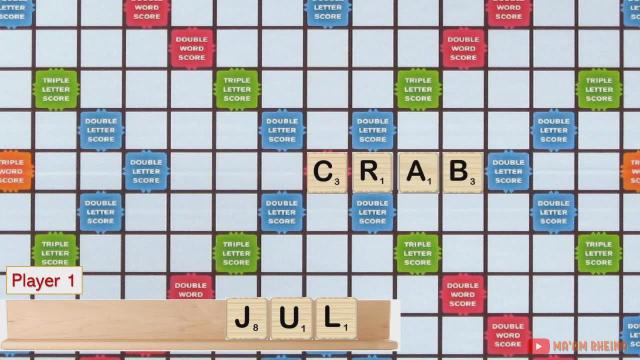 Multiply the total points by two, His score is sixteen. Remember that the center star square has a double word score. Remember that the first player can place a word either across or down. After placing his tiles, the player must draw an equal number from the bag to maintain the 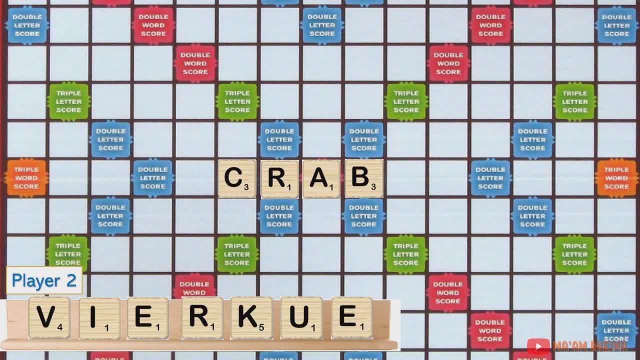 seven tiles per player. The next player must connect his word using the existing letters on the board. Player two placed his letter by forming a word vice Letter V has four point and it is on the triple letter score. Multiple the letter value by three, Then add the remaining. 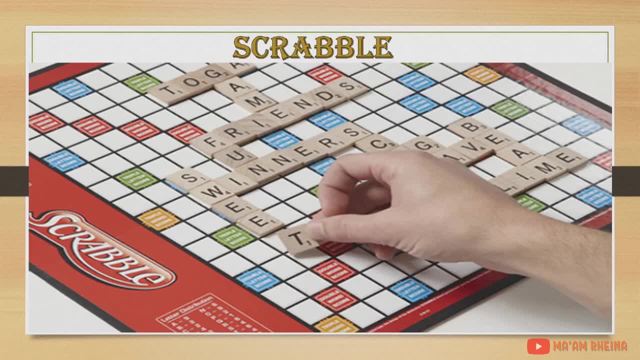 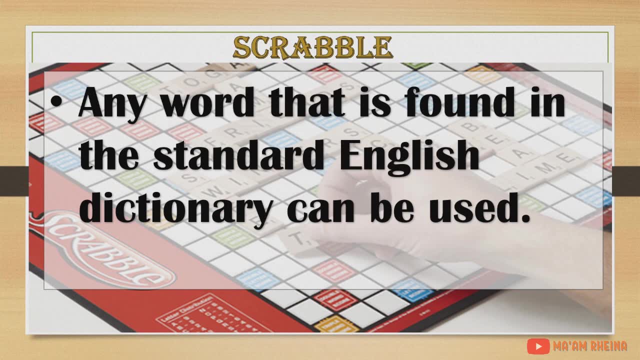 numbers. Player two's score is seventeen. Play continues in a clockwise direction. Any word that is found in the Standard English Dictionary can be used in the game. There are words that are not allowed in the game. This includes suffixes, prefixes. 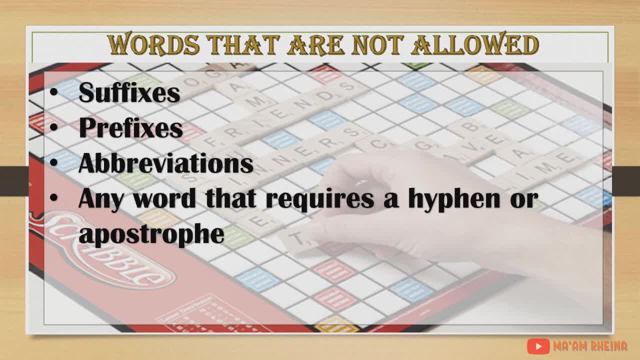 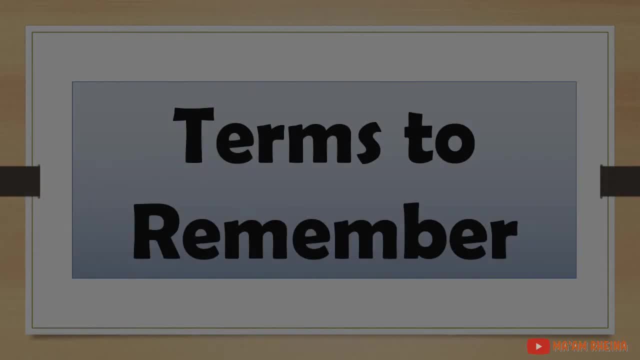 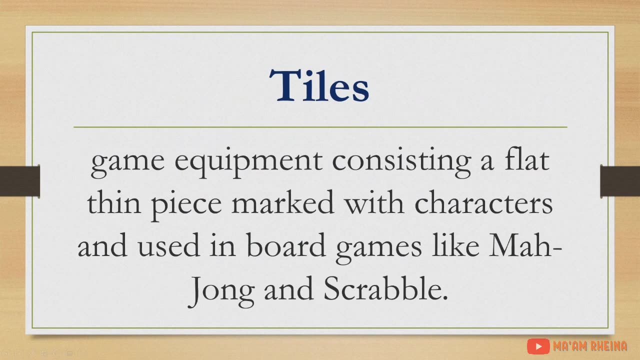 and abbreviation. Any word that requires a hyphen or apostrophe cannot be played in the game. Any word that requires the use of a capital letter. Now let us move on to the terms that we need to remember in playing. Scrabble Tiles- Game equipment consisting of flat, thin piece marked with. 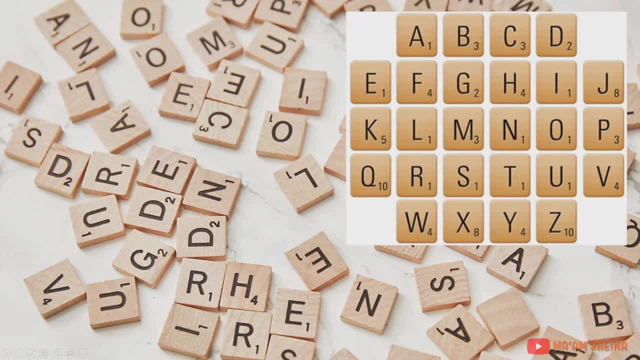 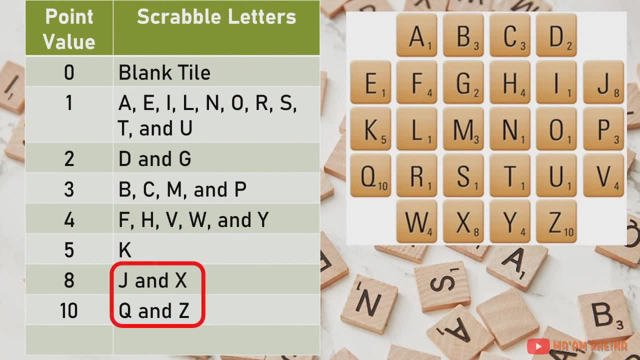 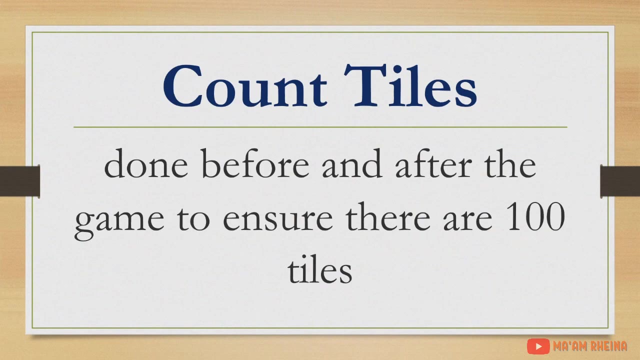 characters and used in board games like Mahjong and Scrabble. Each letter has a point value. J and X has eight points, Q and Z has ten points. Letters J, X, Q and Z are called power tiles, Count tiles. It is done before and after the game to ensure there are one hundred tiles. There should. 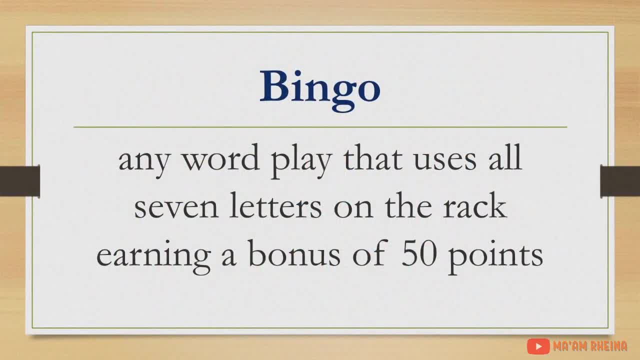 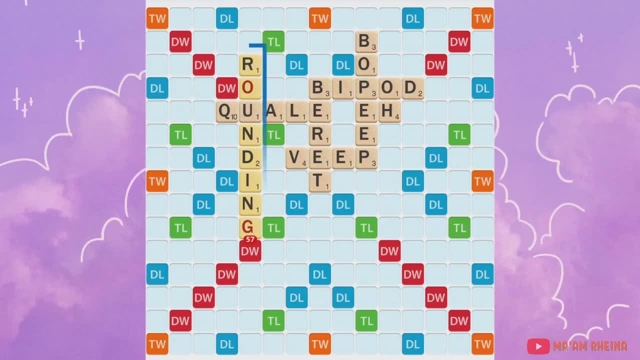 be a total of one hundred pieces of tiles. Bingo: Any word play that uses all seven letters on the rack, earning a bonus of fifty points. Here is an example: There were two blank tiles assigned as O and G. All the seven tiles of the player were used. 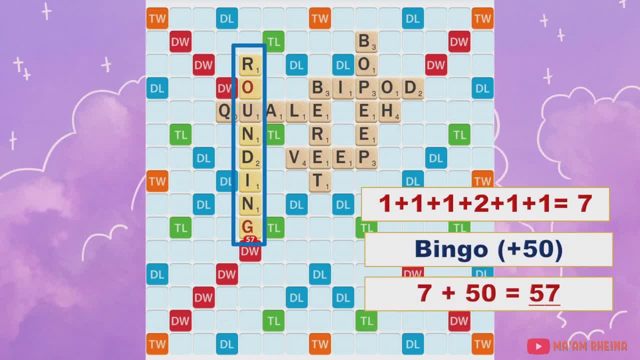 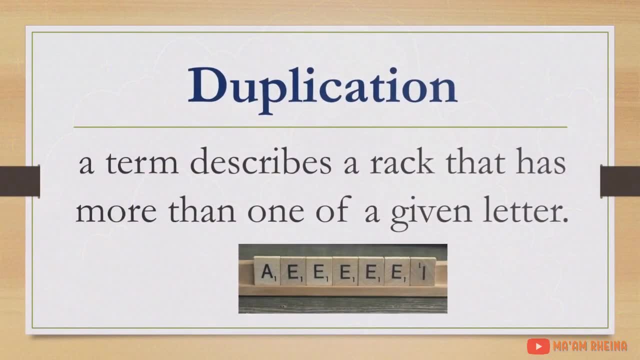 Add fifty bonus points to the word score Bingo. He got fifty-seven. If you own a blank tile that is being used for, you can take the blank tile back by substituting your tile for the blank on the board. Duplication A term describes a rack that has 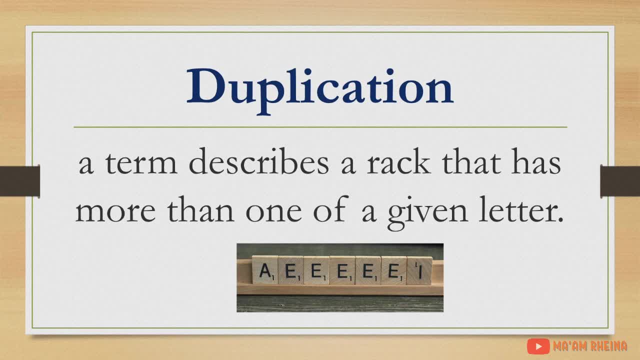 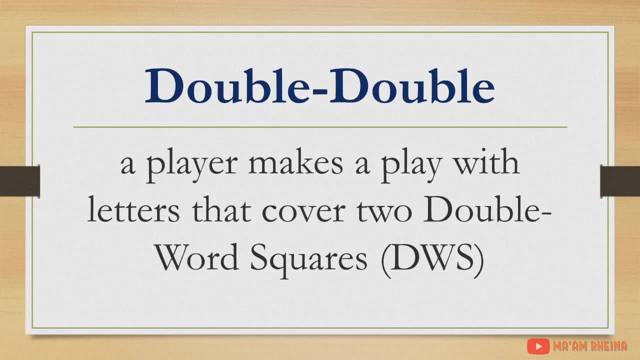 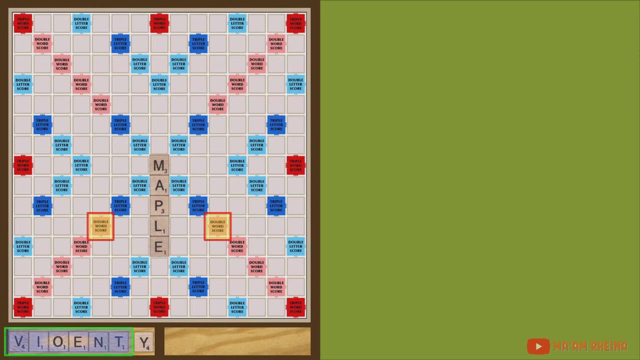 more than one of a given letter. You may exchange your letters but you cannot do anything on that turn. Double-double letters that cover two double word squares. this is an example. to get the double double, you need to get the squares. at that same time, a player now placed a new word, violent, covering the two double. 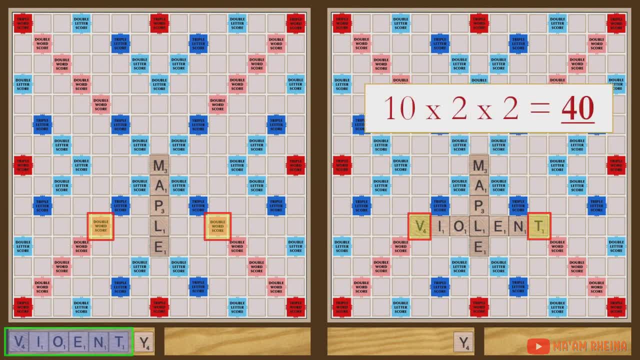 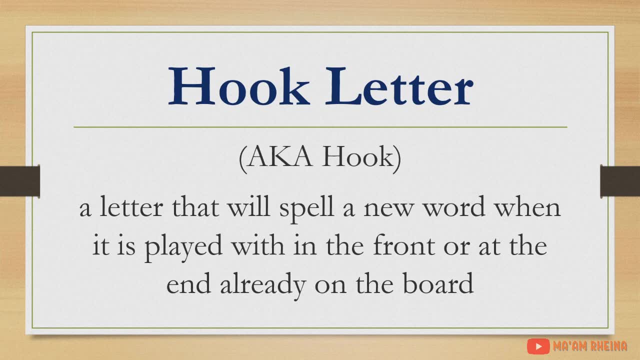 word score. double the word score twice by multiplying the sum of the word score by two. two times double. double hook letter, also known as hook, a letter that will spell a new word when it is played within the front or at the end, already on the board. an example is by putting 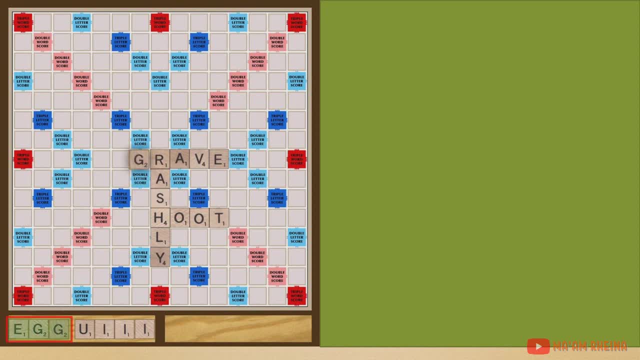 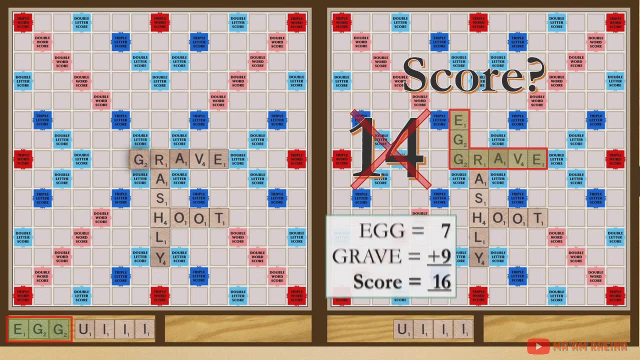 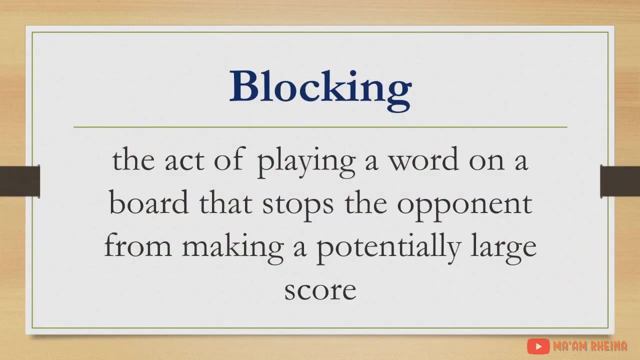 letter g before the word rave. this player can make more than one word by placing the word egg. what will be his score if your answer is 14? try again. he made two word at the same time: one score for egg and another for grave. his total score for this turn is 16.. blocking the act of. 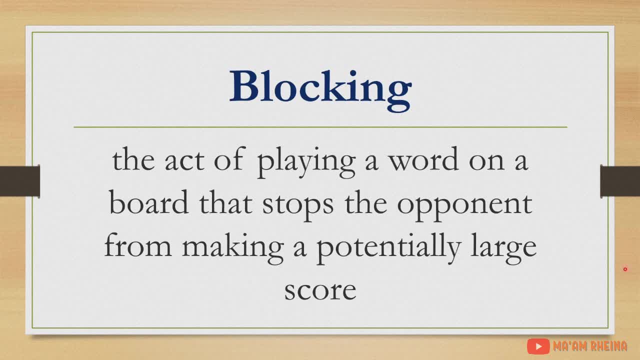 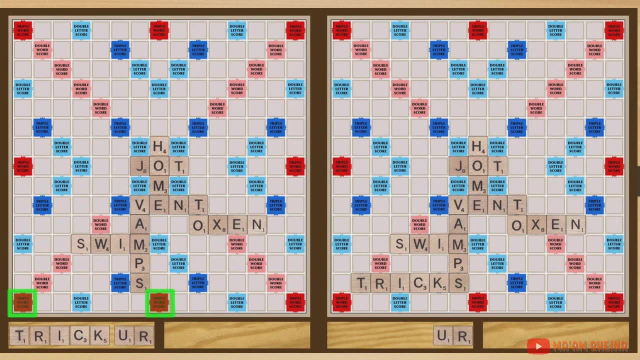 playing a word on a board that stops the opponent from making a potentially large score. if you cannot have these triple words scored during your turn, think of a strategy so others cannot have these triple words scored during the turn. triple word scored as well. Challenge: When a play is not acceptable. 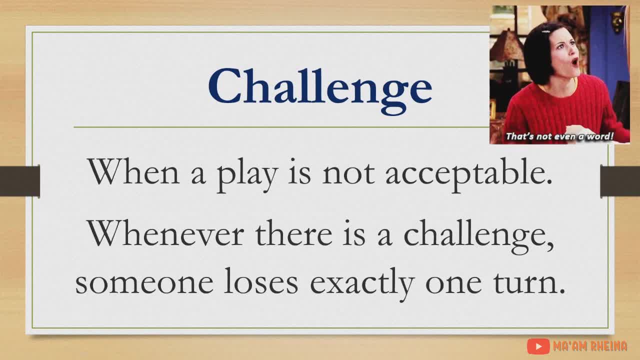 You can only use a dictionary when there is a challenge. Whenever there is a challenge, someone loses exactly one turn. If the word is not in the dictionary, the player losses their turn. If the word is allowed, the challenger loses their turn. 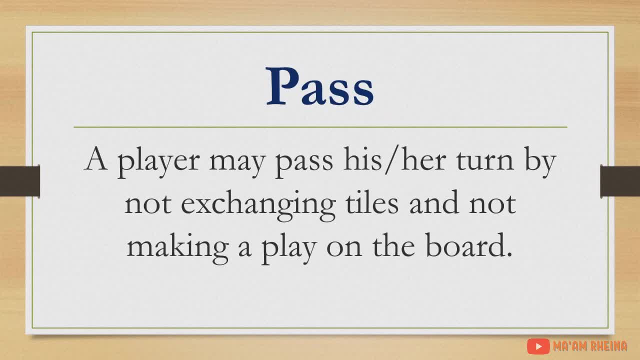 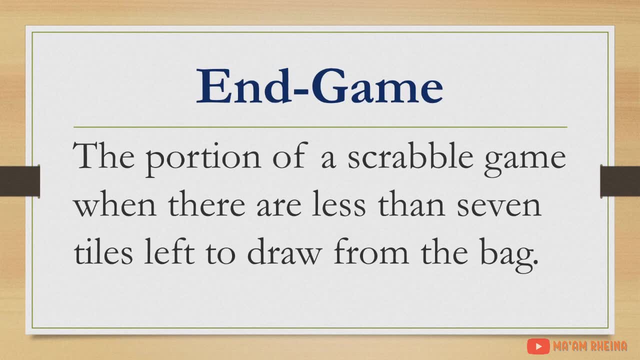 Pass. A player may pass his- her turn by not exchanging tiles and not making a play on the board. End game- The portion of a Scrabble game when there are less than seven tiles left to draw from the bag. When no one can make any more words, the game ends. 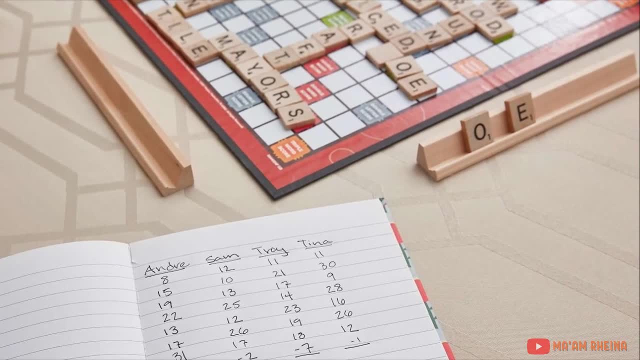 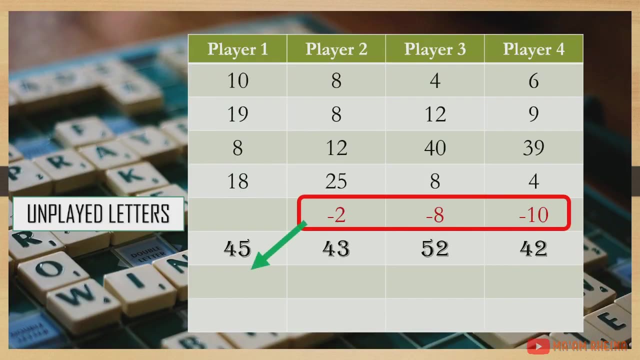 Calculate each player's final score by adding up the points from all of their word scores. If there were unplayed letters, subtract it to their total points. If one player has used up all of their letters, add the sum of everyone else's unplayed. 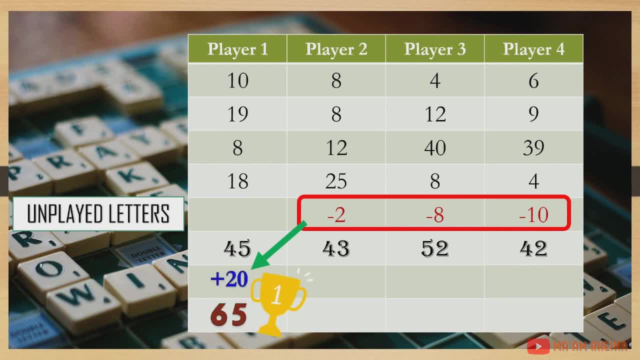 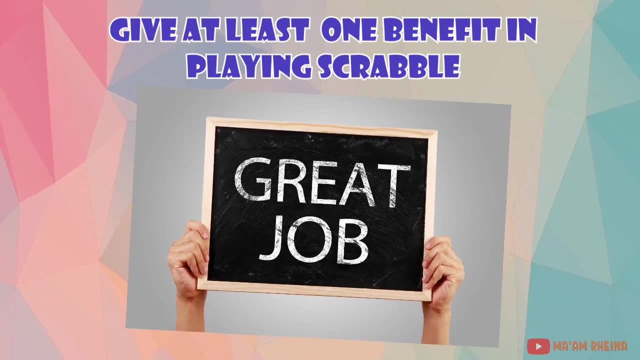 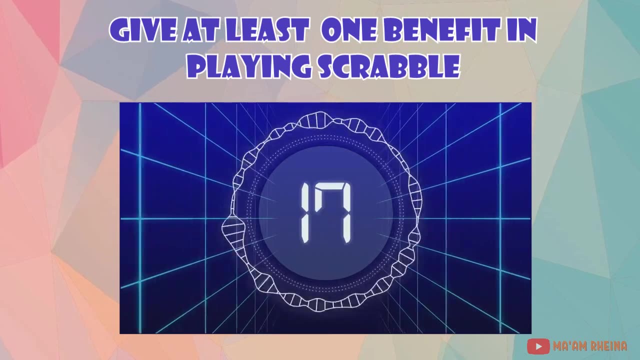 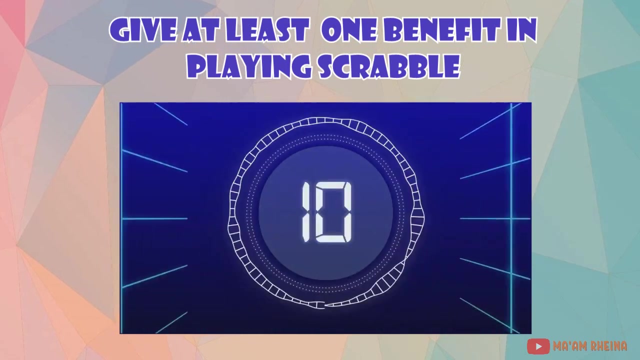 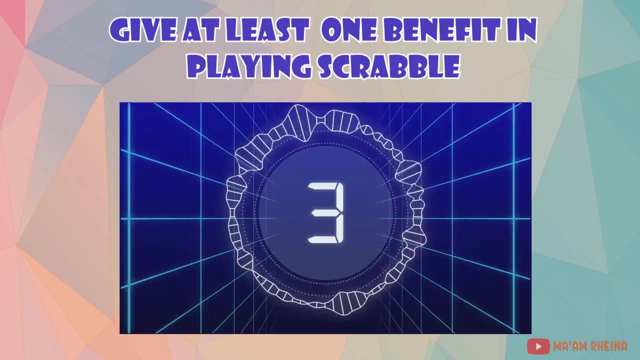 letters to their score. The player with the highest score wins. There you have it. In the comments section, write at least one benefit in playing Scrabble. I will give you 20 seconds to decide. Just type your answer. Now let us answer the next exercise. 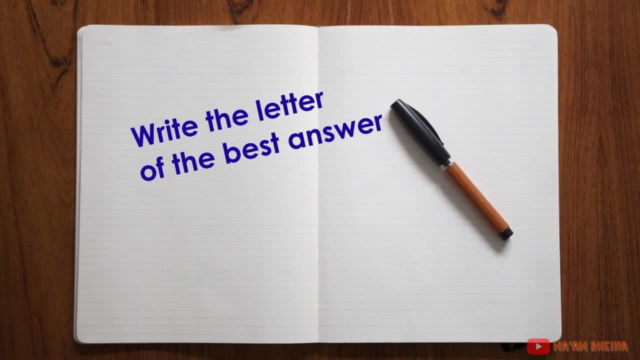 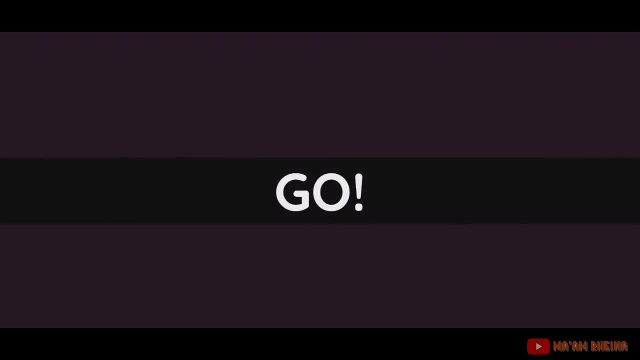 Grab a paper and pen, choose the best answer and write the letters. only This exercise will help you to understand the order of the game. The order of the game is very simple: Draw the numbers from each row. Each row has a number. 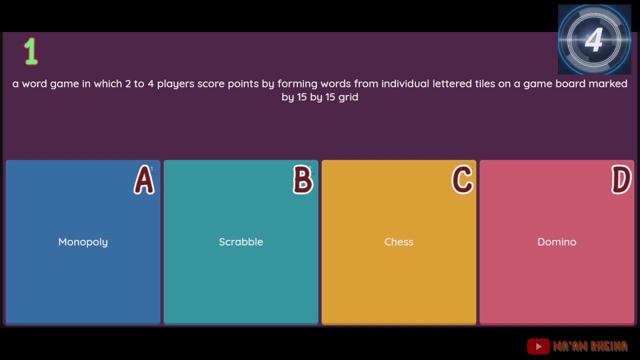 In these groups of words. you can apply the sum of your letters Today. I will draw a number based on one of the numbers on each row. Try to guess the number based on your answer. If you are not sure, let me know in the comments. 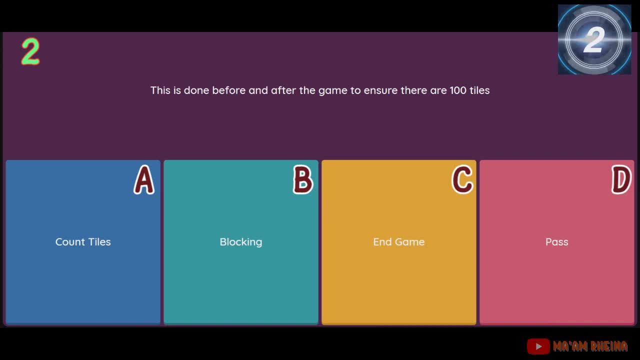 Try to guess which number is the number that you want to draw. It is very easy, And if you fail to guess the answer, you will have to do some more tests. Let's start with the move. Play a game, Thank you. 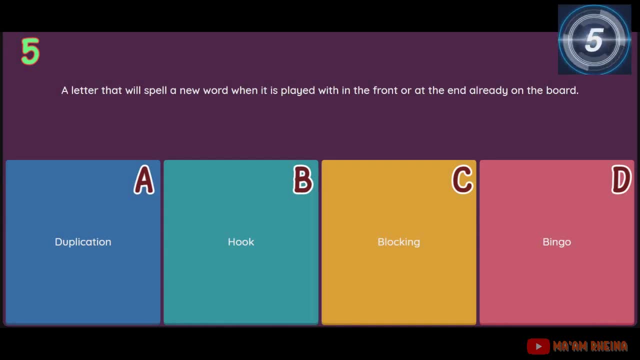 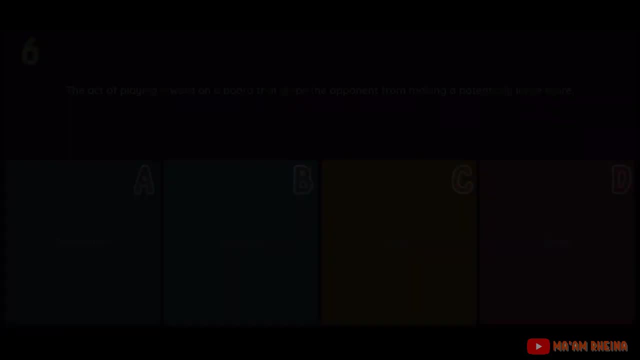 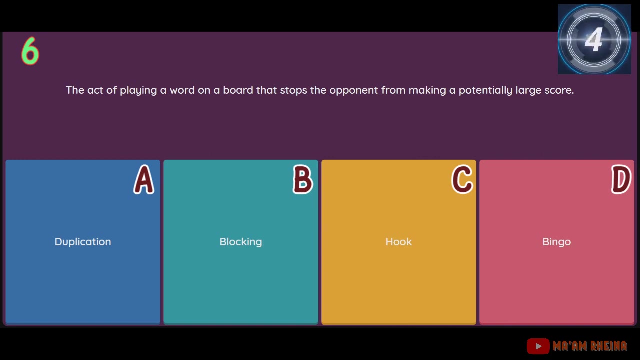 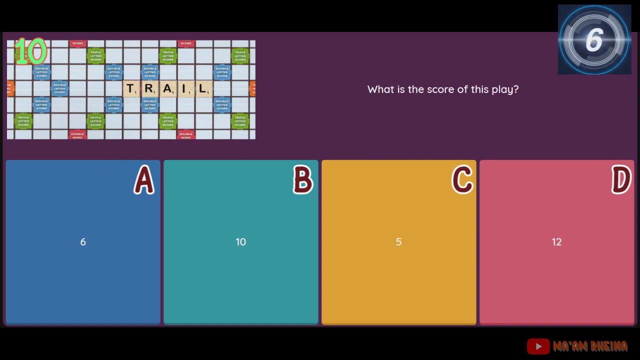 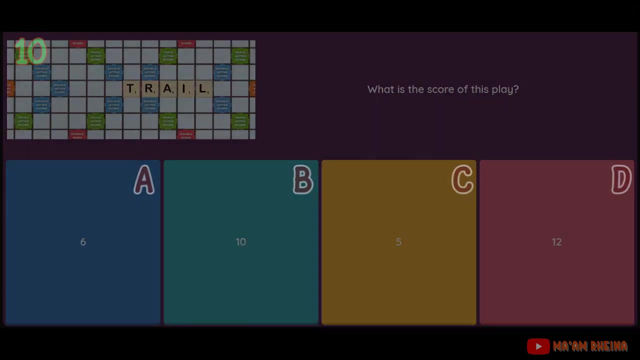 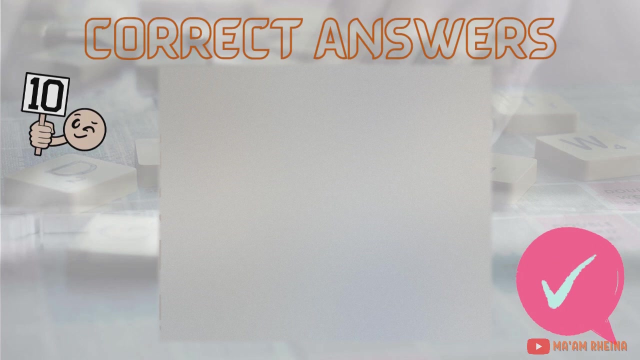 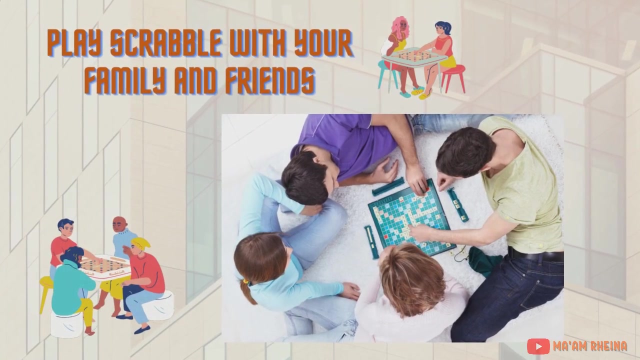 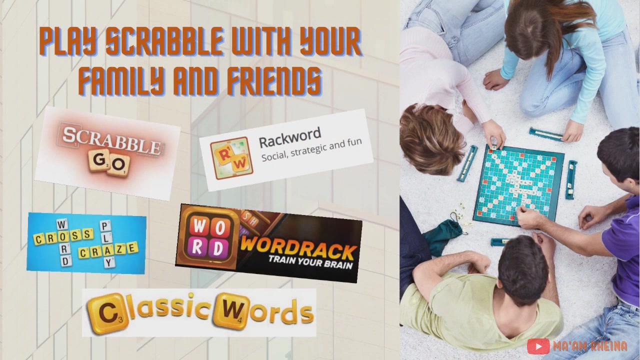 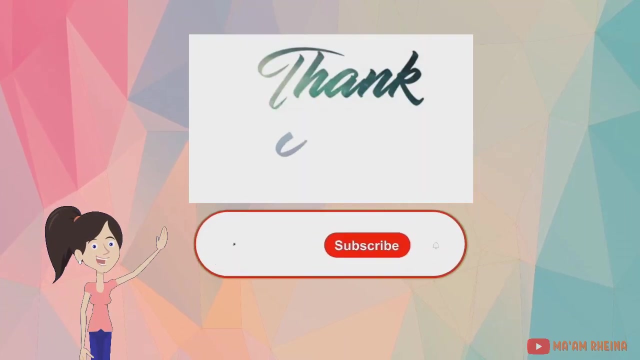 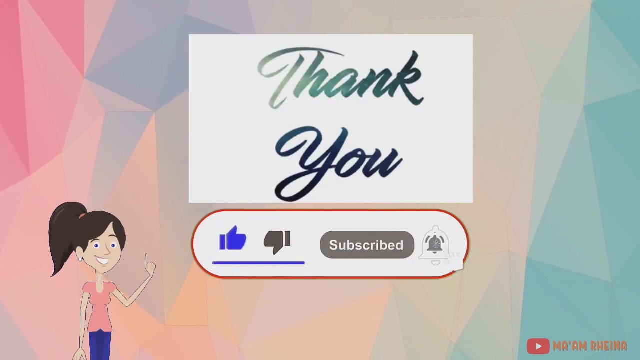 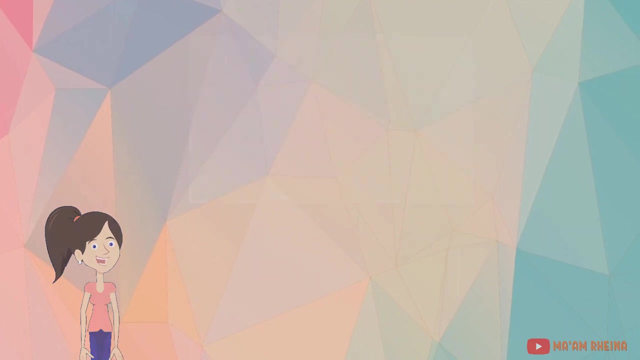